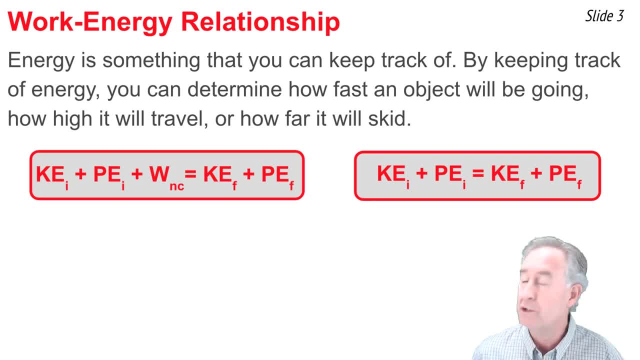 will go and how far it will skid. In this video we'll be using these equations here along the way. Let's begin with three others. First, the kinetic energy equation that Ke is equal to one half mass times speed squared. The equation for gravitational potential energy is that: 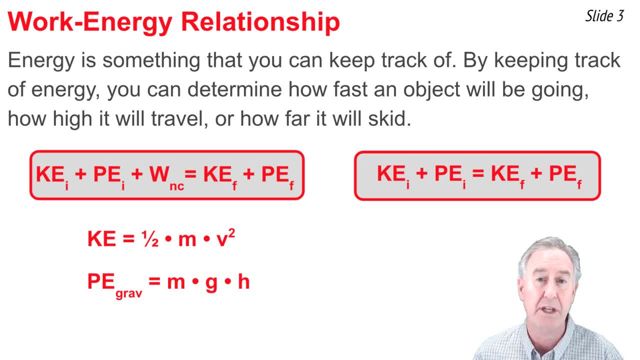 Pe grav is equal to mass times g times the height. G here is 9.8 newtons per kilogram on planet earth. And finally we need the equation for work done by non-conservative forces. You take that force, you multiply by the displacement of the object and by the. 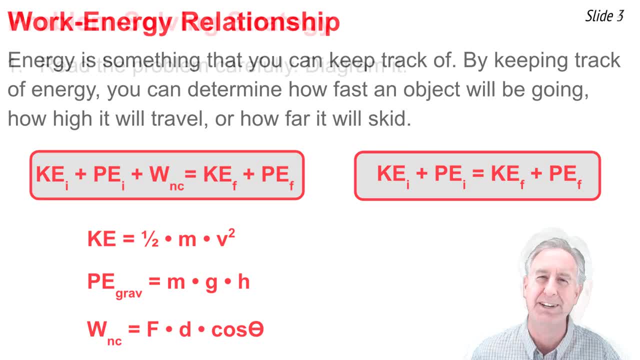 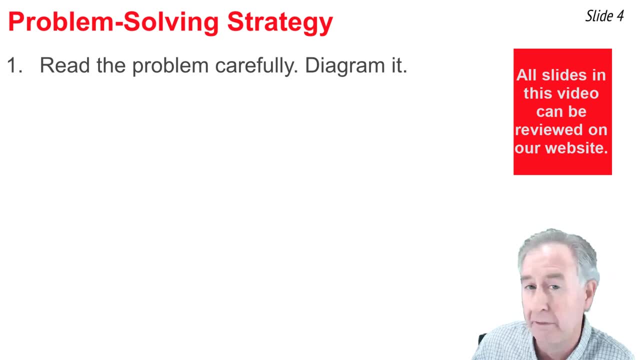 cosine of the angle theta between the force and the displacement vector. Let's discuss a problem solving strategy for how to approach these problems. The first step is to read the problem carefully, Get a mental picture of what's going on. It helps to diagram it. The second step is to look for numerical values within the problem. These: 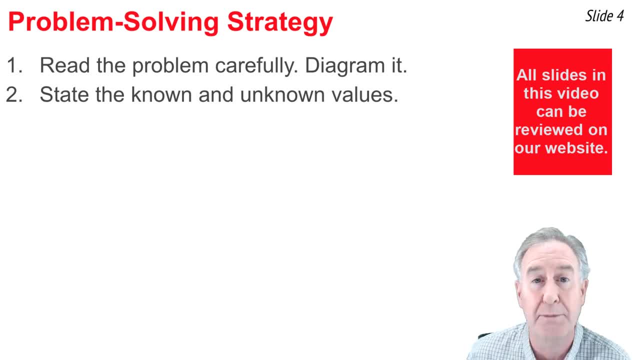 are the knowns? Identify what they are by writing them down and relate them to symbols within your equation. For instance, say something like HI equal 21.7 meters. Also, identify what the unknown value is. what you're looking for. It might be something like VF- equal question. 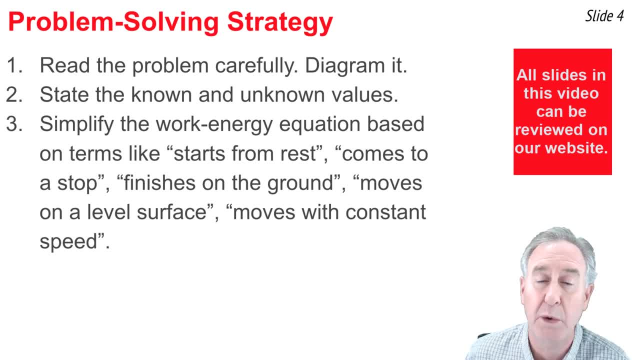 mark. The third step is to simplify your work. energy equation- Turn that five term equation into a simpler form. Look for terms like starts from rest and comes to a stop, moves across level ground or moves with a constant speed, in order to simplify terms that are zero or 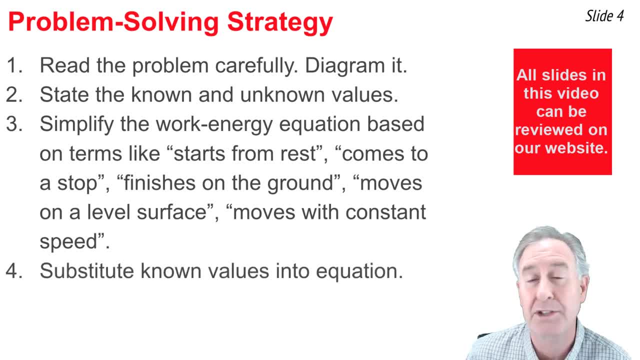 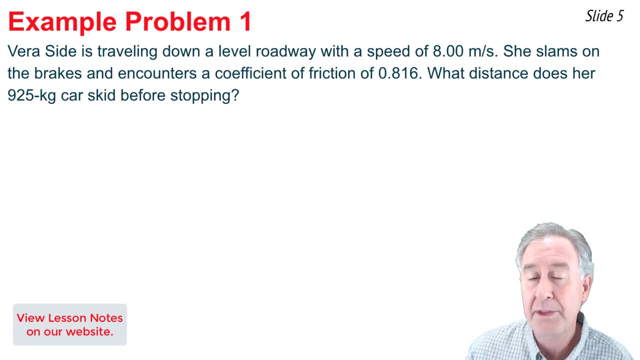 are the same on both sides of that equation. The fourth step is to take the numerical values that you know and substitute them into the equation, Then perform the necessary algebra steps in order to solve for the unknown. The first example problem is about a 925 kg car that's moving at 8 meters per second. 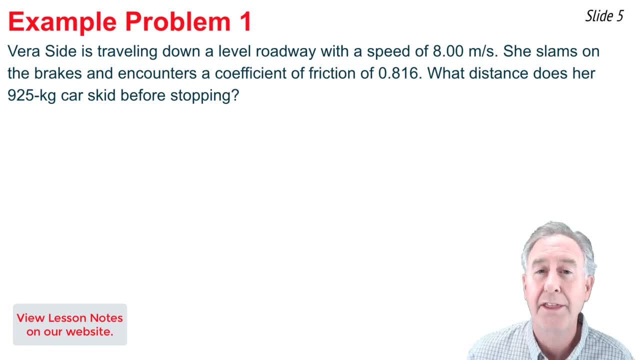 along a level highway and skids to a stop. The coefficient of friction, mu, as we call it, is .816, and we want to know what distance does it skid before stopping. So when I go to write down my known values, I'm going to write down the initial speed and the final. 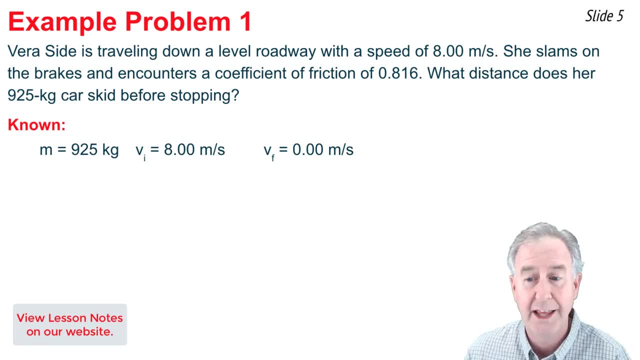 speed and the mass values, and I'm going to write it like that. I'm also going to write down the value for mu, the coefficient of friction, and I'm going to write it like that of friction, and I'm going to pay attention to the fact that the road is 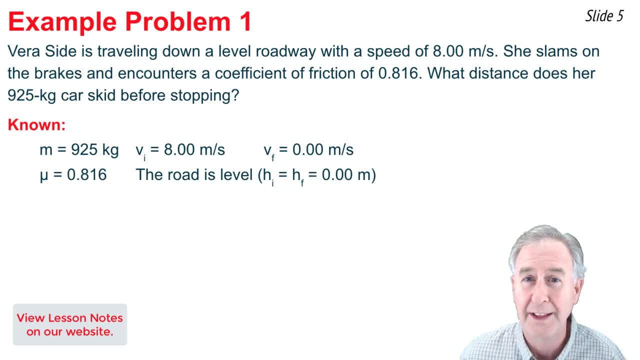 level. so the initial height and the final height are both zero. Now this is what I'm picturing: cars moving along a level highway, initially with eight meters per second. it's got kinetic energy. finally it's stopped no kinetic energy, and I'm looking for the value of D. I'm going to take my equation, my work. 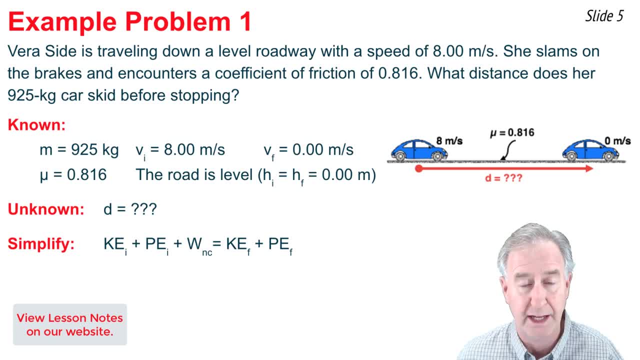 energy equation, this five term equation. I'm going to simplify it by canceling any zero terms. Now the Ke final is zero, it's stopped and the initial potential and the final potential are both zero because it's on the ground. So I now have 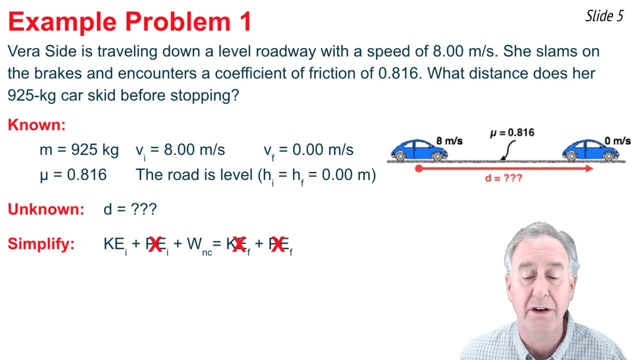 a two term equation, Kei plus W and C equals zero. I'm going to take the Kei and expand it to say one half mvi squared, because that's how we'll be calculating it, and for W I'm going to go the force of friction times D, times the cosine of. 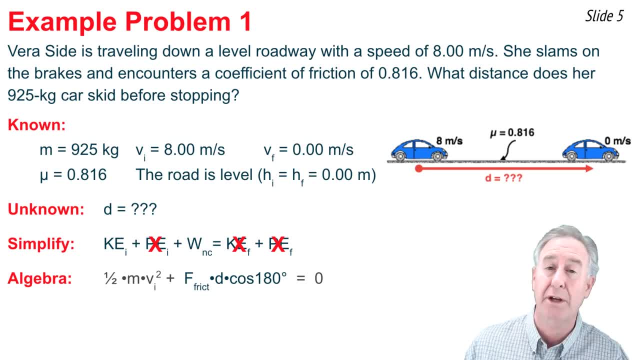 the angle between the F and the D. Now in this diagram the car is moving to the right and friction acts to the left, So the force vector is left, the displacement vector is right and the angle between opposite directed vectors is 180 degrees. So I substitute that into this equation. The 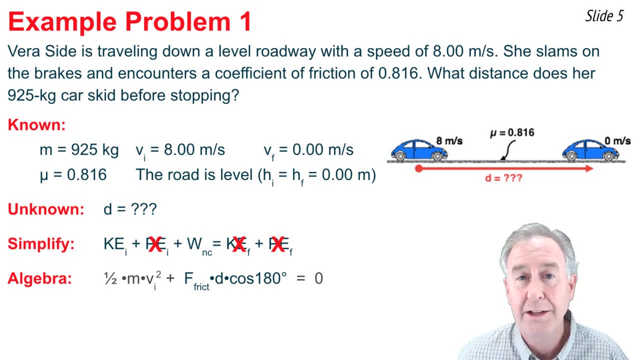 right side is zero. Now for the force of friction. it's always mu F norm. that's from another unit and on a level surface. the normal force from the surface is equal to the gravity force on the car. So F friction is equal to mu times the. 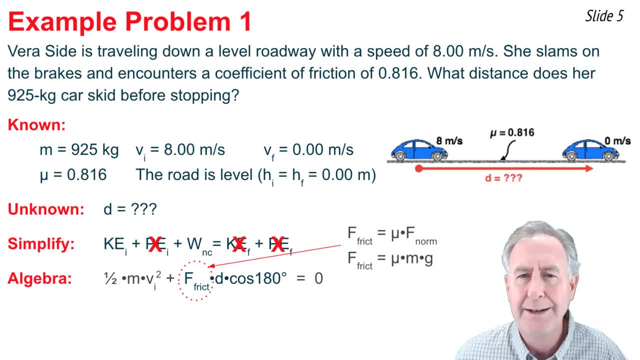 gravity force or mu times mg. Now pay attention to that cosine of 180 there. If you don't know what it is, try it on your calculator: It's negative one. So that second term is actually a negative term because of the cosine of 180 and I. 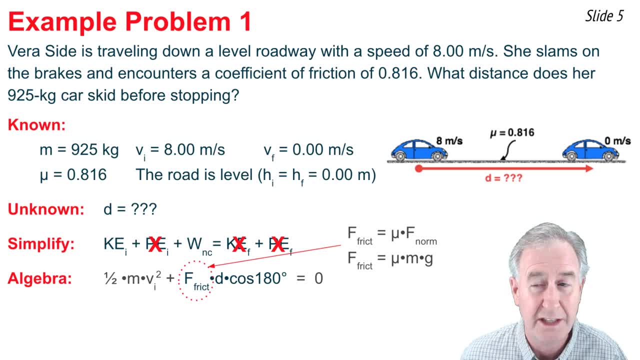 can swing it around to the right side of the equation and make it positive, and that's what I've done in this next step, along with substituting values into the equation like 925 for m and 8 for v, and I have over, on the other side, the point. 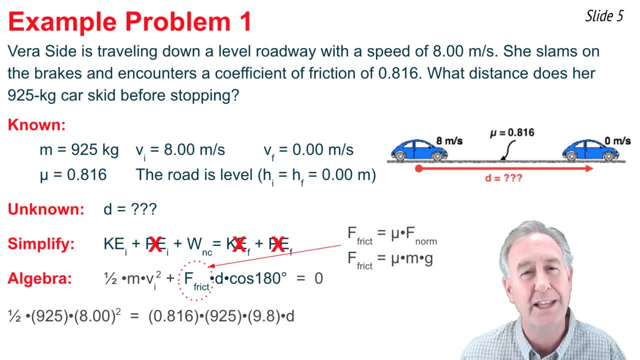 816 for mu and the 925 for m and the 9.8 for the value of G. I'm looking for D, One equation, one unknown. Pull out your calculator, evaluate the left side, then evaluate everything in front of the D on the right side and write it down Now. 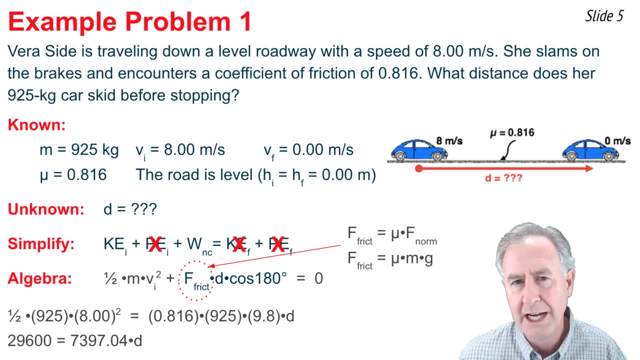 you're solving for D. So what you want to do is divide both sides of that equation by the 7397 figure, and when you do you'll get the value of D. Do it on your calculator. It comes out to be a little short of 4.. In fact it rounds to 4.00. 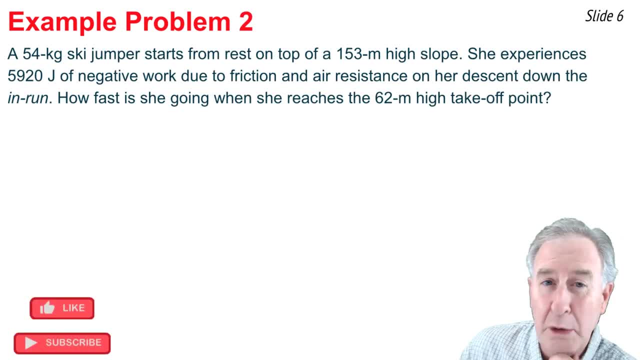 meters. In our second problem we have a 54 kilogram ski jumper starting from rest at a known height of 153 meters high. It goes down the slope towards the takeoff point and we know at takeoff point it's 62 meters high and we know that there's. 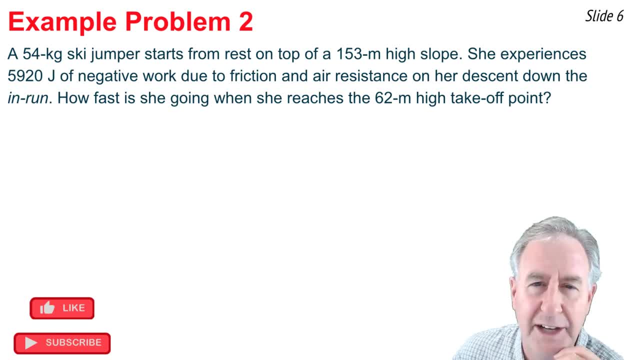 work done by friction and air resistance. We know the amount: It's negative 5920 joules. We want to know how fast is this person going at takeoff? So when I write what I know, I'm going to list the mass, I'm going to list the initial speed at 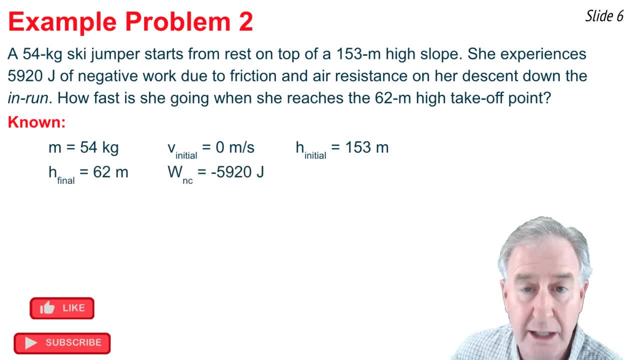 zero. I'm going to list the initial height. I'm going to list the final height. I'm going to list this negative work value done by friction and air resistance. I'm picturing this situation with work being done along the slope and it's negative. 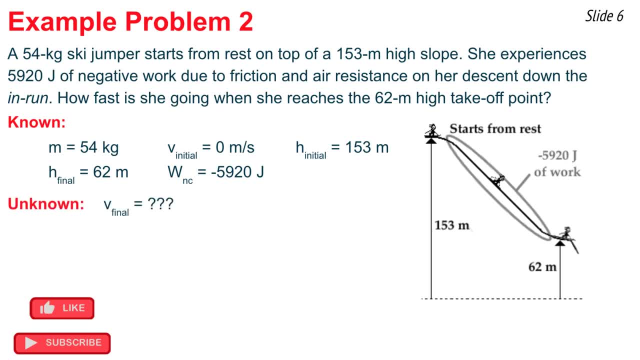 work. What do I want to know? I want to know how fast is it going? That's a V value, The VF, The final velocity at takeoff point. So I'm going to take my equation and I'm going to simplify it. 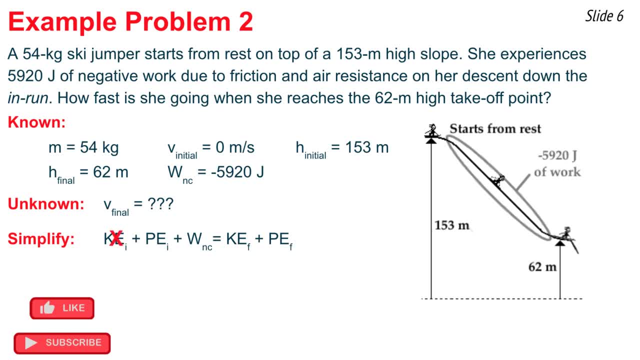 That five term equation cancels to four. when I figure that the initial kinetic is zero, The ski jumper starts from rest. Now I'm going to take that equation and I'm going to expand it to use the variables like one half mv, squared and mgh's, And I have this equation. Now what I'm going to do is I'm going to 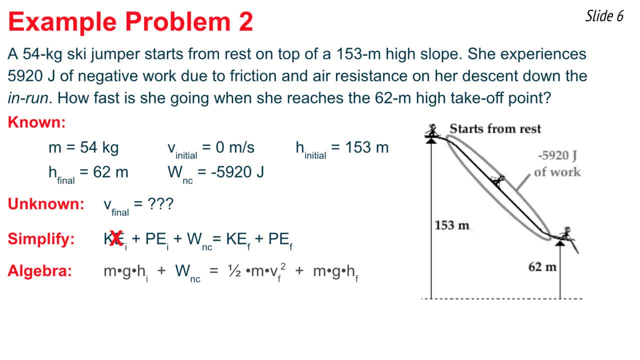 substitute my known values. I have them all listed there. I just bring them down and insert them where they belong, And when I do, it looks something like this: Now there's a one half 54 times V final squared. That simplifies to 27 VF squared. Everything else there can be calculated on your. 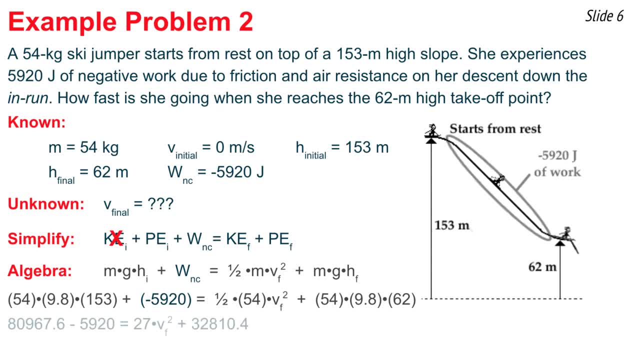 calculator Find out what they are. Then, when you're done, you should have something that looks like this: And take that 32810 term, which is on the side with 27 VF squared, Subtract it from both sides so it cancels from the 27 VF squared. 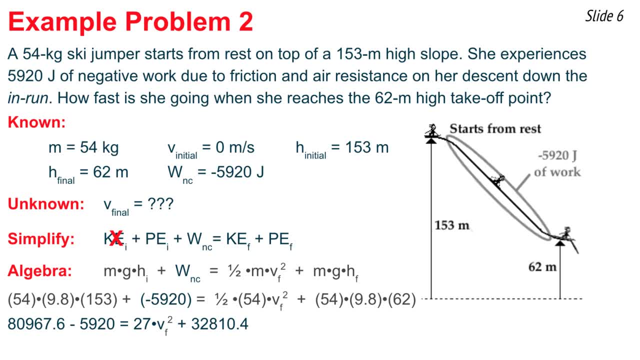 side And that's by itself And it ends up on the other side. Use your calculator to evaluate what 808967 and negative 5920 and negative 32810 is. It comes out to be this: And now know, 27 VF squared is equal to 42237.. Divide both sides by the 27 and 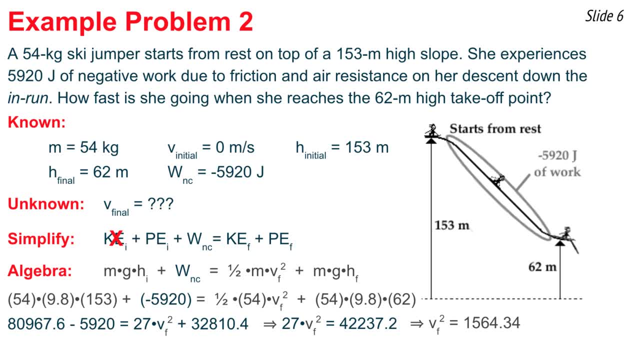 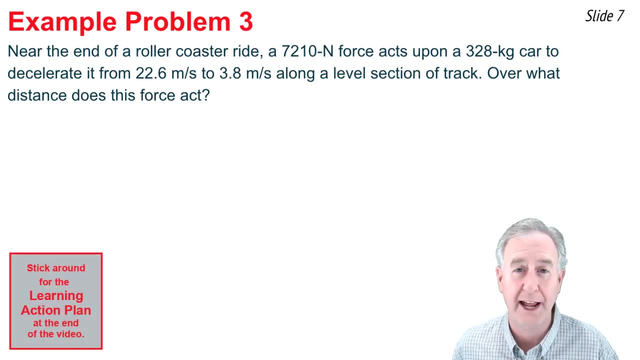 you end up with VF squared is 1564 and some change. Take the square root of both sides and you get something like 39.55 rounded to two significant digits here, And it's 40 point meters per second. Example three is about a roller coaster car moving along a level track and 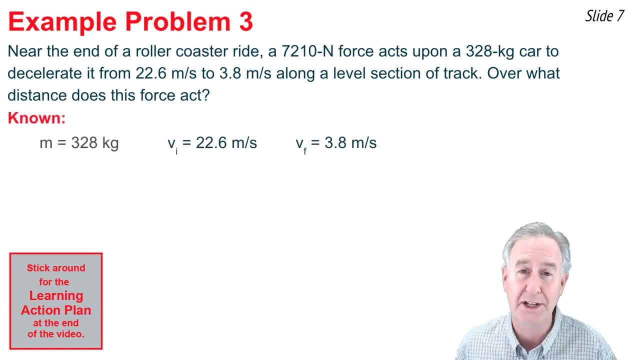 slowing down When I ask: what do I know? Well, I know the mass, I know the initial speed, I know the final speed, I know the force that acts upon the car And I know the track is level. So HI is equal to HF, which is equal to zero. I'm picturing. 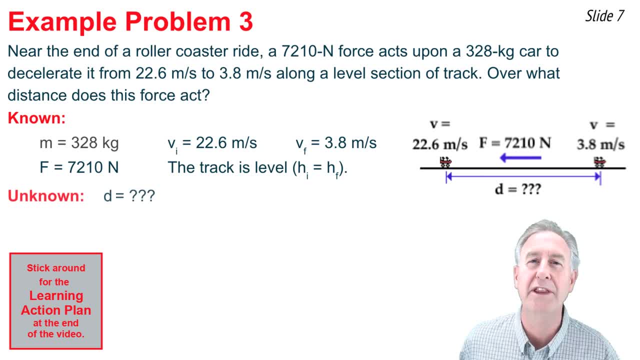 something that looks like that. What am I looking for? The distance between that initial speed and final speed location. I take my work energy equation and I simplify it, And when I do, I use the fact that the track is level and the car is on the track. So both terms are zero. They cancel from the equation. Now I 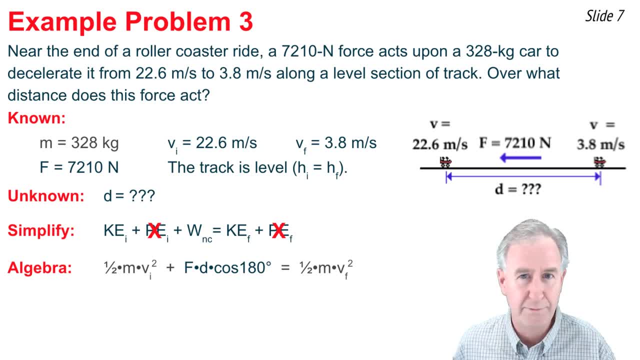 expand each term in this three term equation with 1 half MV squared and FD cosine theta, And you'll notice that the cosine of theta is cosine of 180 degrees because the object, the roller coaster car, is moving to the right, But its force is 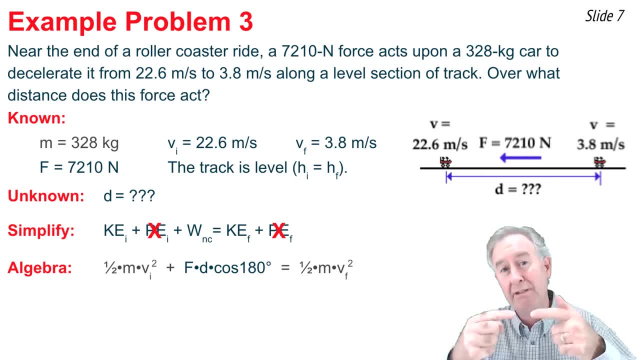 against it to slow it down. So the angle between the F and the D vector is 180 degrees. Now I'm going to substitute known values into this equation And it looks something like that. You'll notice that that second term on the left side. 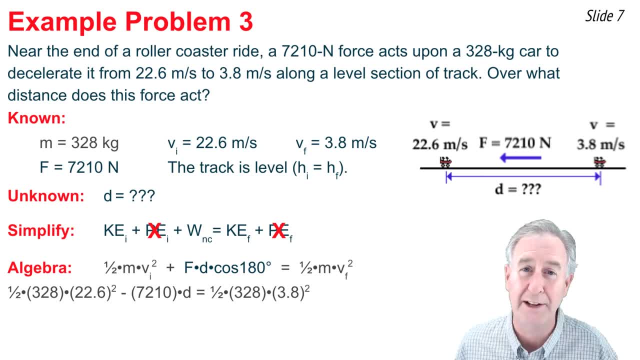 becomes negative because the cosine of 180 is negative 1.. Now what I want to do is pull out my calculator and evaluate each of the terms- The first term and the third term- And it turns into something like this: Now I'm going to get the 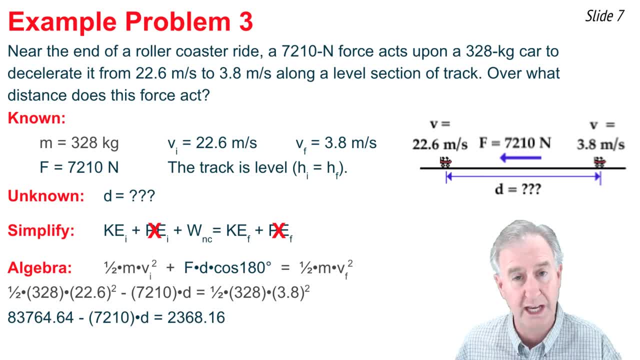 7210D term by itself, And the way I'm going to do that is add it to both sides of the equation And I'm going to subtract the 2368 from both sides of the equation And I end up with something that looks like this: I'm trying to solve for D, So I divide both. 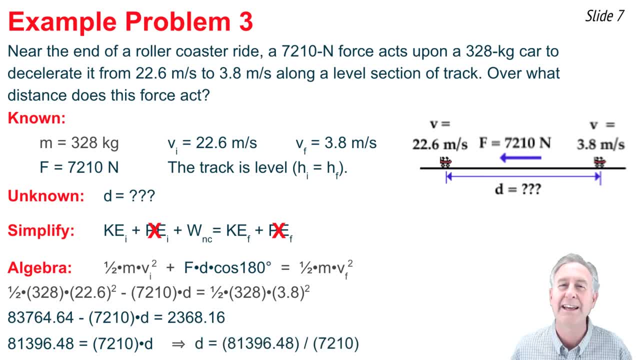 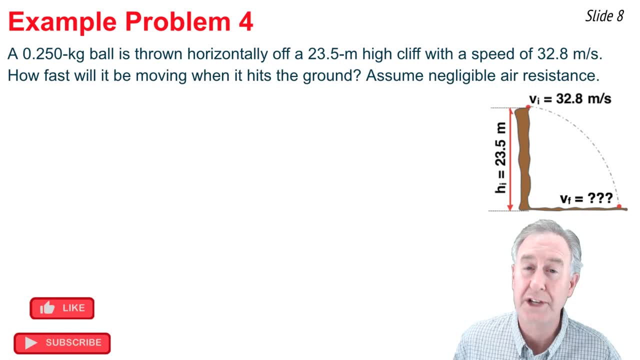 sides of the equation by 7210.. I pull out my calculator and find out what that is, And it's about 11 meters. Example 4 is about a ball that is launched horizontally from the top of a tall cliff, And I'm picturing something that looks like that. What I know is I know the mass of the. 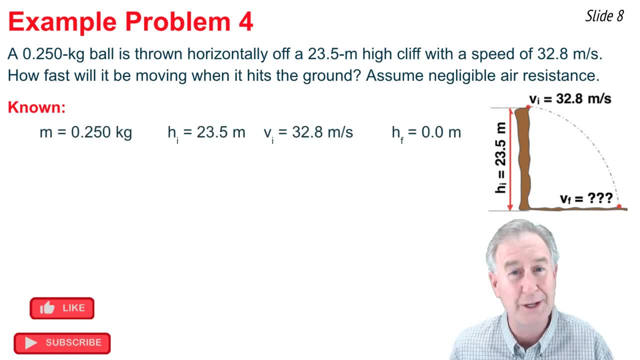 ball and the height initially, And I know the height finally, And I know the initial speed And what I'm looking for is the final speed. I'm told to assume negligible Resistances forces. So I go to take my work energy equation to simplify it And I 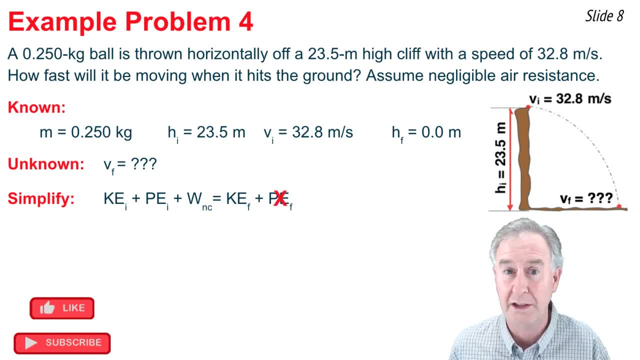 recognize that the PEF is zero And I also recognize that the only force doing work is gravity. It's a conservative force, So W and C is equal to zero. Now I have a three term equation And I'm going to expand each term with the formula for K and PE. So it looks. 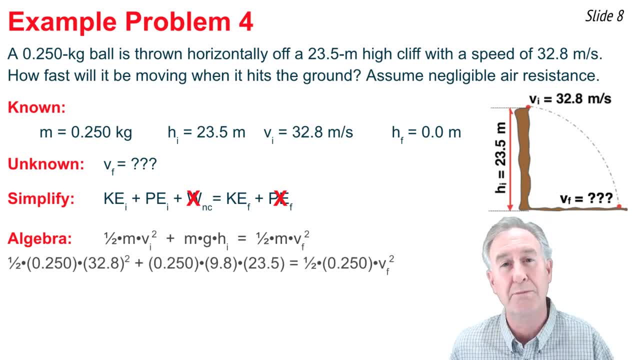 something like this And substitute known values in for mass and heights and speeds, And I have this situation. I'm going to pull out my calculator and evaluate and simplify. each term of the equation Turns it to this And I have this VF squared term over on the right side I'm looking to find 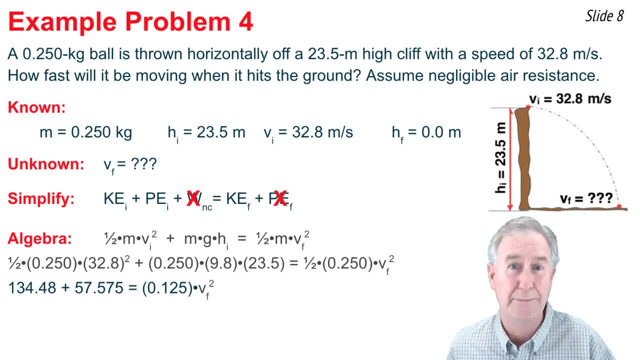 out what VF is. So I'm going to do two algebra steps in one here. I'm going to take the two terms on the left side and add them together, Combine them And then divide through both sides by 0.125.. When I'm done I got this. VF squared is equal to the 1536 figure Now. 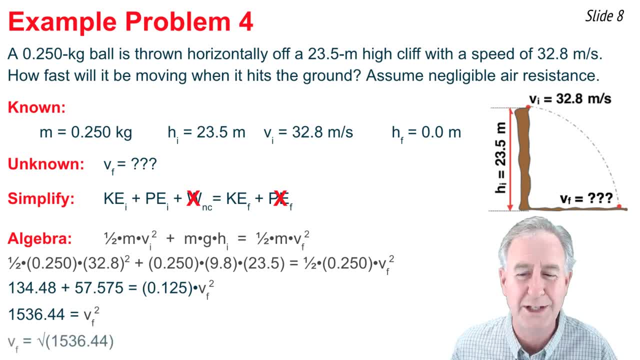 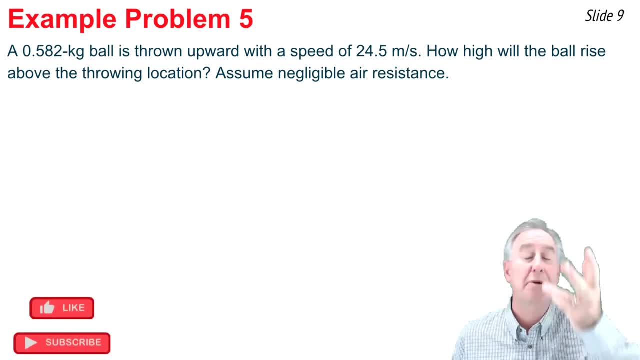 if you don't want to know what VF is, you must take the square root of both sides, And when you do, you end up with 39.2 meters per second. In example five, a ball is thrown upwards And I know its mass and its initial speed. 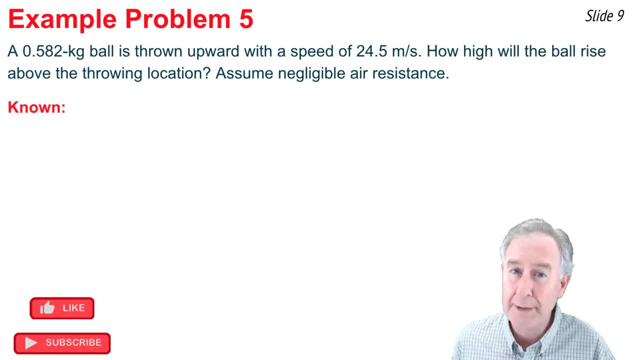 And I want to know how high it will go. So when I ask, what am I given? I'm given the mass value, I'm given the initial height, the zero. I'm given the initial speed of 24.5.. And I know that when it's at its highest point it will have momentarily run out of that speed. 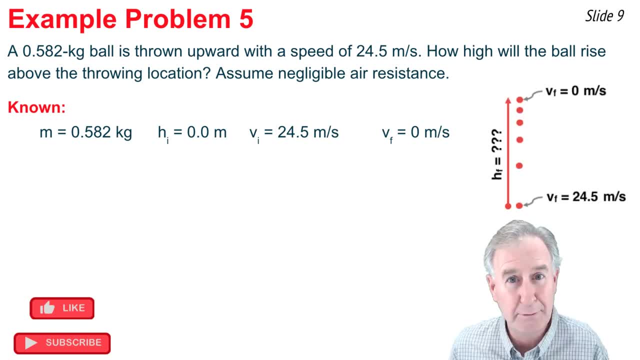 And it will be a final speed of 0 meters per second. What am I looking for? I'm looking for the final height. How high does it go? Now I take my work, energy equation, and I simplify it. I know that the initial PE is zero. It starts from zero height, And I know that when 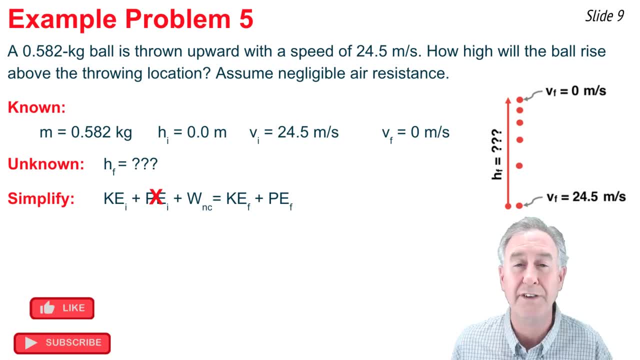 it reaches its highest point, it's not moving. So the kinetic energy, finally, is zero, And the only force doing work on this ball is the force of gravity. That's a conservative force, And so the W and C is equal to zero. 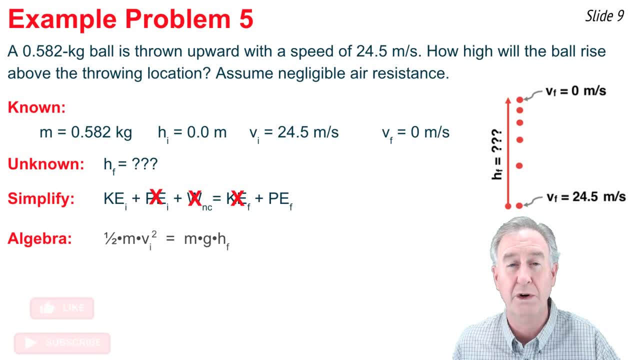 I have a two-term equation. I can expand it with the formulas for Ke and Pe, And then I can substitute in known values of M, V and G. And I have this equation. Pull out your calculator and simplify both sides, And then you're looking for HF. So divide through. 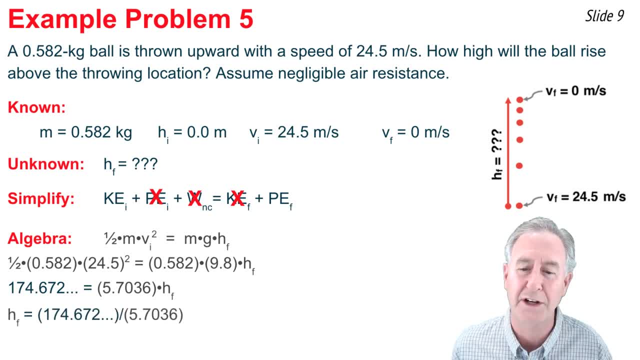 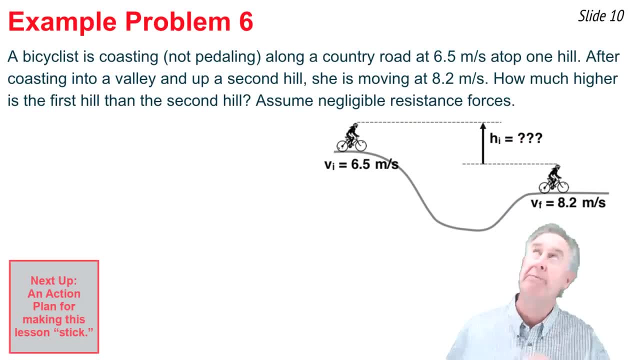 both sides of the equation by this 5.7036 figure And when you're done, you have the final height of 30.6 meters. In my sixth and final problem, I have this situation of a bicycle. I have a bicycle that's coasting, not pedaling, on top of one hill And then it goes into. 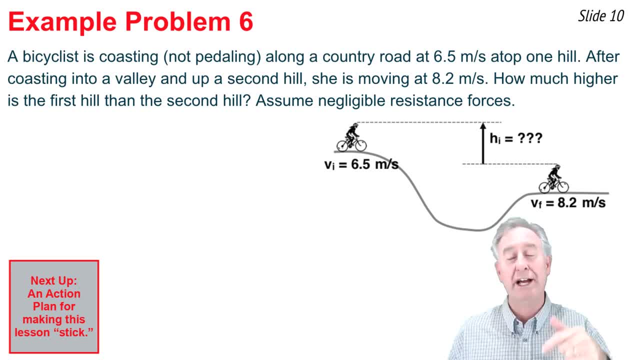 the valley up on top of a second hill And I want to know how much higher is the first hill than the second hill. So when I ask, what do I know? I know the VI and I know the VF And I'm going to try to find what is the height of the first hill if I call the second hill. 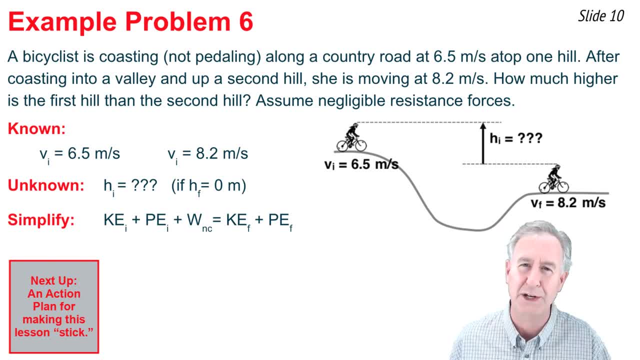 a zero height. I'm looking for HI, given that HF is zero. I take my work energy equation and I simplify it. I cancel out the P, I take the VEF term, since HF has been declared zero, And the W and C term is zero as well. 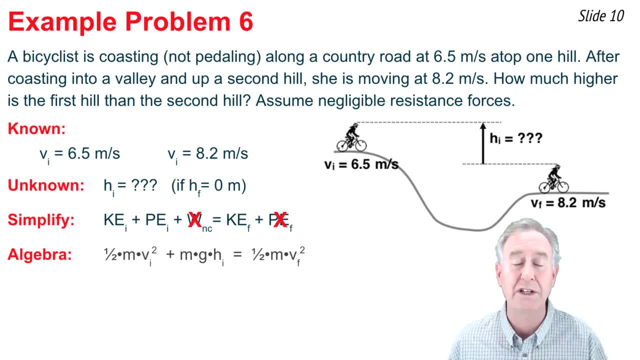 since the only force doing work is the force of gravity, a conservative force. Now I'm going to take the term, the three energy terms, and write the expression 1, half mv, squared and mgh in for them. And at this point I'm getting ready to substitute. but 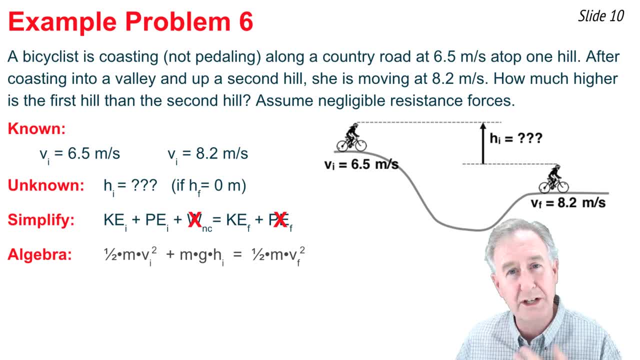 I don't know my mass, But if you look at the equation there's an m in each term. So if you were to divide through every term of the equation by m, you'd still have an equation, But then in my function I'd have an equation that my mass is equal. And if the mass is,